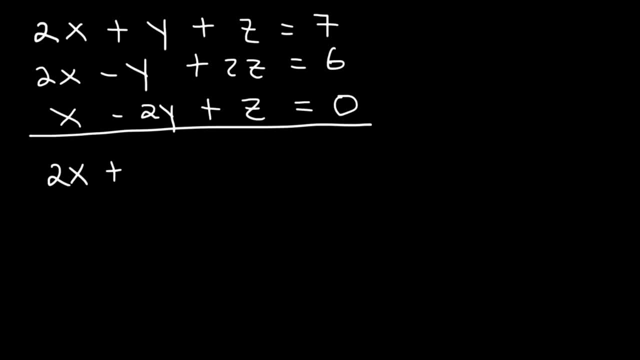 So first I'm going to rewrite it. So once we add them, 2x plus 2x is 4x, z plus 2z is 3z, and 7 plus 6 is 13.. Now I'm going to save this equation. 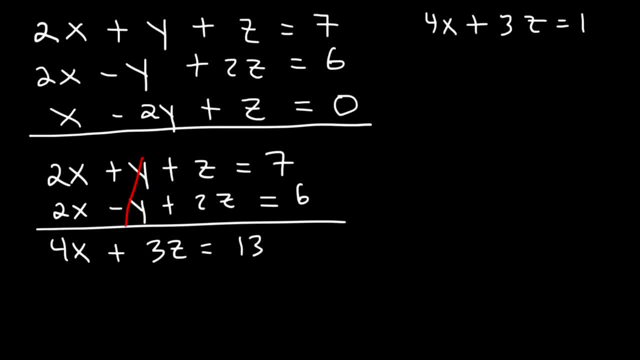 Now what we need to do next is we need to combine another two equations and cancel the same variable, y, But we need to include equation 3, because we didn't use it. We only used the first two equations. We can use equation 1 and 3, or 2 and 3.. 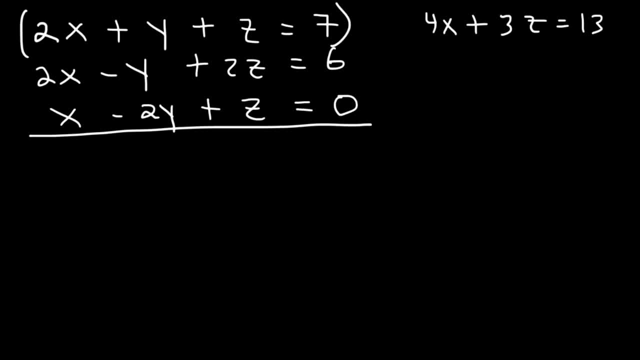 Let's use 1 and 3.. To cancel y we need to multiply the first equation by 2.. So 2x times 2 is 4x, y times 2 is 2y, z times 2 is 2z. 7 times 2 is 14.. 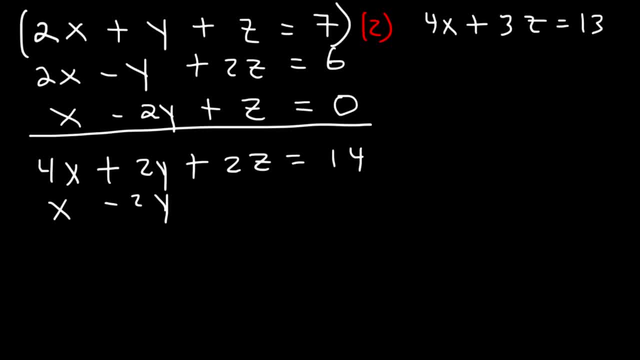 Now let's rewrite this: We have the third equation right beneath the modified first equation, And let's add them 2y and negative. 2y cancels. 4x plus x is 5x. 2z plus z is 3z. 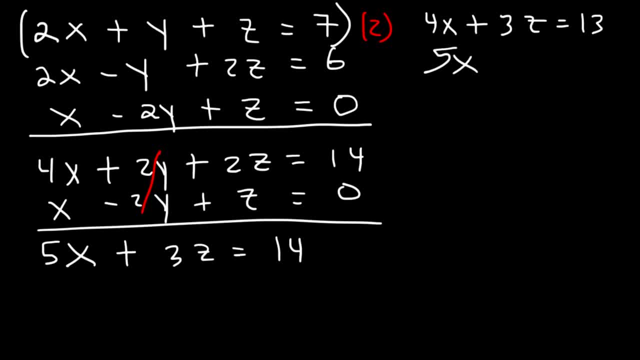 So here's the second equation that we have in terms of x and z: 5x plus 3z is equal to 14.. Now to solve those two equations, we just need to multiply one of them by negative 1.. Let's multiply the first equation by minus 1.. 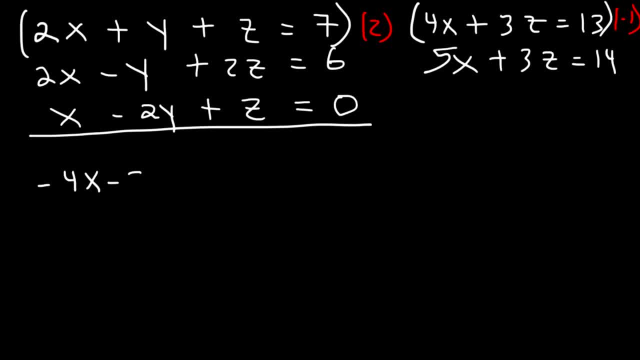 So it's going to be negative 4x minus 3z, which is equal to negative 13. And let's rewrite the other equation right beneath it. So let's add the two equations So we can see that z will cancel. 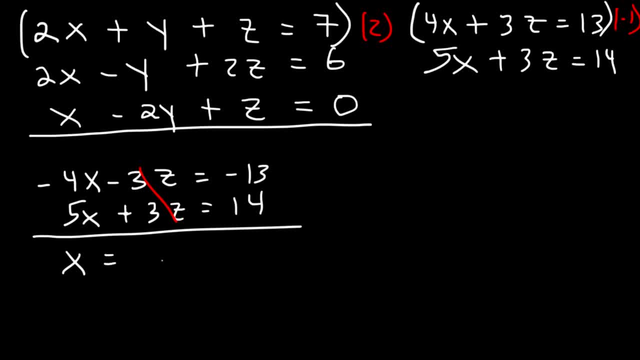 Negative 4x plus 5x is 1x. Negative 13 plus 14 is 1.. So therefore, x is equal to 1.. Now let's plug that value into the first equation- Well, not the first equation, but the second equation in terms of x and z. 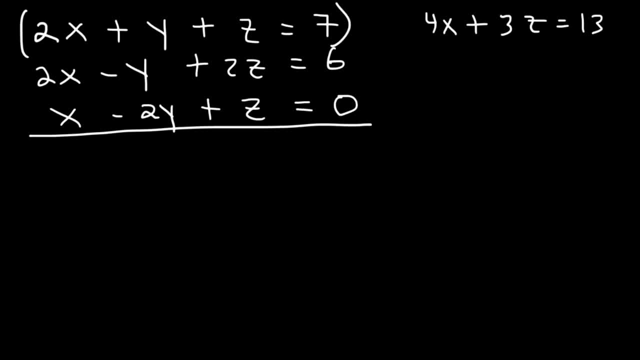 Let's use 1 and 3.. To cancel y we need to multiply the first equation by 2.. So 2x times 2 is 4x, y times 2 is 2y, z times 2 is 2z. 7 times 2 is 14.. 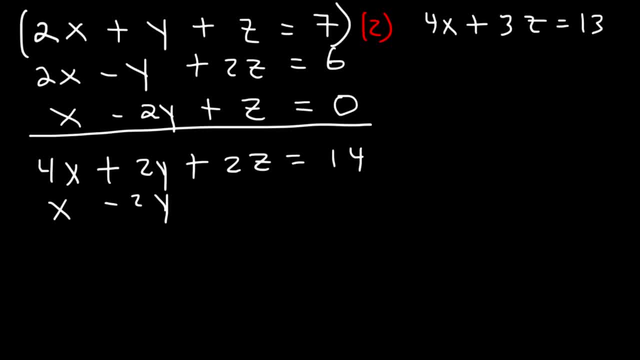 Now let's rewrite this: We have the third equation right beneath the modified first equation, And let's add them 2y and negative. 2y cancels. 4x plus x is 5x. 2z plus z is 3z. 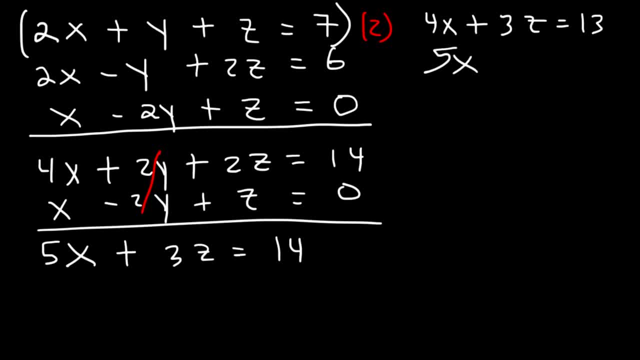 So here's the second equation that we have in terms of x and z: 5x plus 3z is equal to 14.. Now to solve those two equations, we just need to multiply one of them by negative 1.. Let's multiply the first equation by minus 1.. 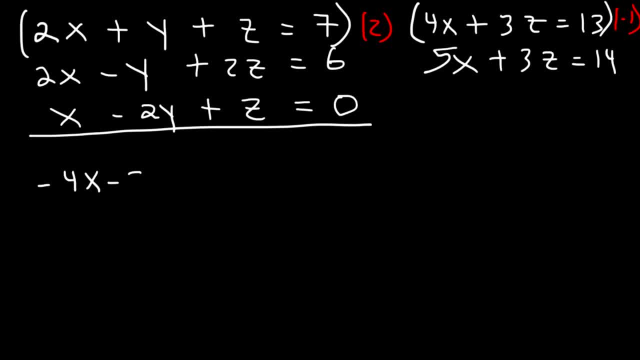 So it's going to be negative 4x minus 3z, which is equal to negative 13. And let's rewrite the other equation right beneath it. So let's add the two equations So we can see that z will cancel. 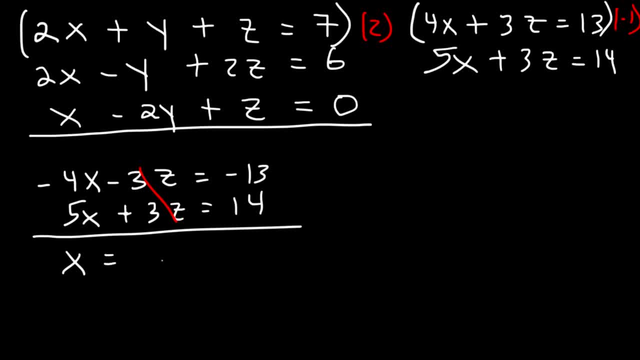 Negative 4x plus 5x is 1x. Negative 13 plus 14 is 1.. So therefore, x is equal to 1.. Now let's plug that value into the first equation- Well, not the first equation, but the second equation in terms of x and z. 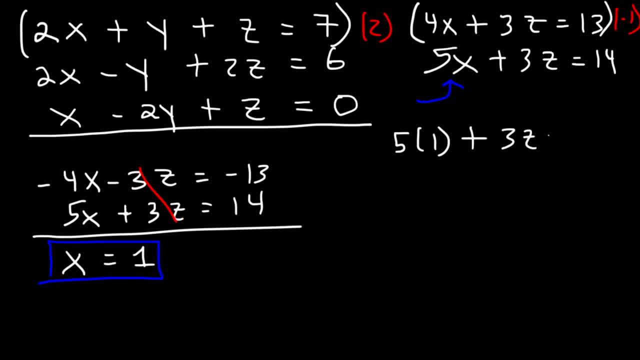 So it's going to be: 5 times 1 plus 3z is equal to 14.. If we subtract both sides by 5, 14 minus 5 is 9.. And then we'll divide both sides by 3.. 9 divided by 3 is 3.. 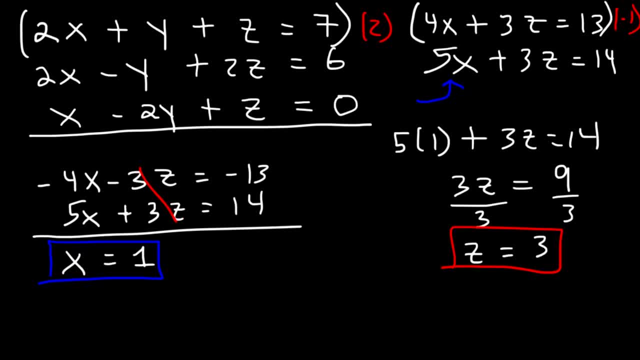 So z is equal to 3.. Now we need to find the value of y. Let's use the first equation in its unmodified state, The original first equation. So x is 1.. We don't know the value of y. z is 3.. 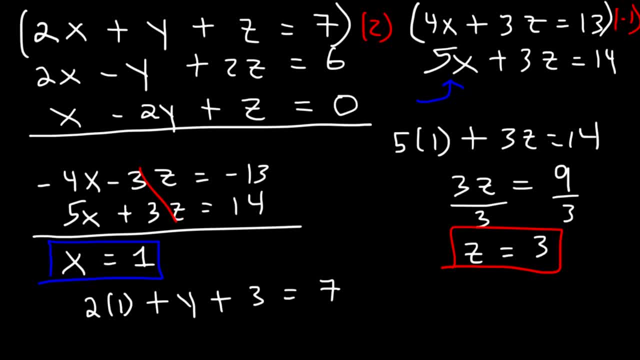 So let's combine like terms: 2 plus 3 is 5.. So y plus 5 is 7.. Now let's subtract both sides by 5.. 7 minus 5 is 2.. So y is equal to 2.. 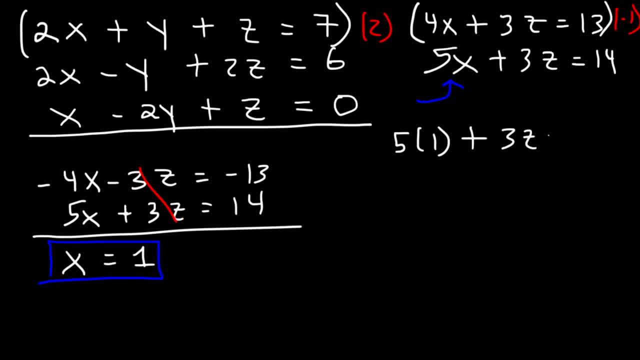 So it's going to be: 5 times 1 plus 3z is equal to 14.. If we subtract both sides by 5, 14 minus 5 is 9.. And then we'll divide both sides by 3.. 9 divided by 3 is 3.. 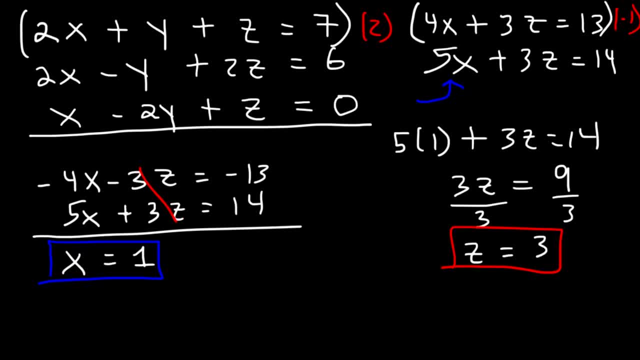 So z is equal to 3.. Now we need to find the value of y. Let's use the first equation in its unmodified state, The original first equation. So x is 1.. We don't know the value of y. z is 3.. 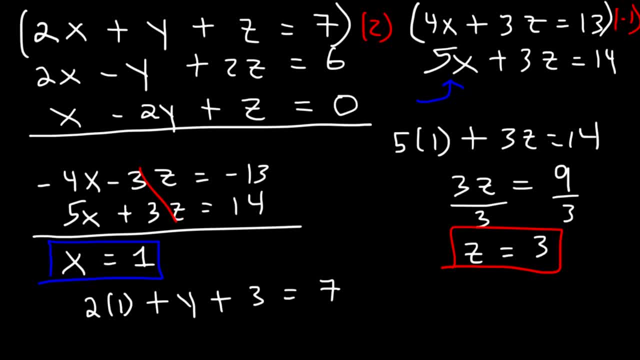 So let's combine like terms: 2 plus 3 is 5.. So y plus 5 is 7.. Now let's subtract both sides by 5.. 7 minus 5 is 2.. So y is equal to 2.. 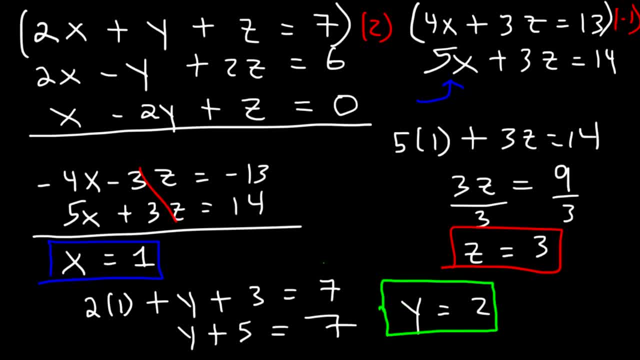 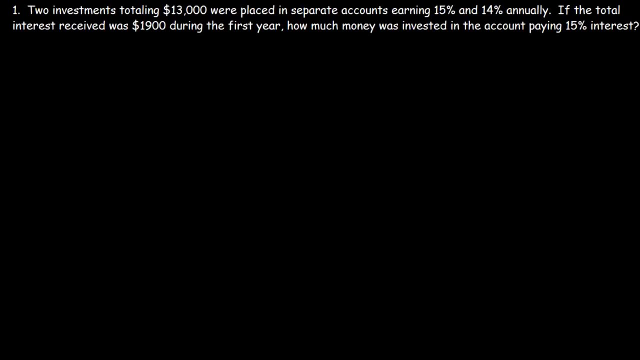 So we can write the answer like this: 1 comma, 2 comma 3.. x, y is z. So that's it for that problem. Now let's work on some word problems. Two investments totaling 13,000 were placed in separate accounts. 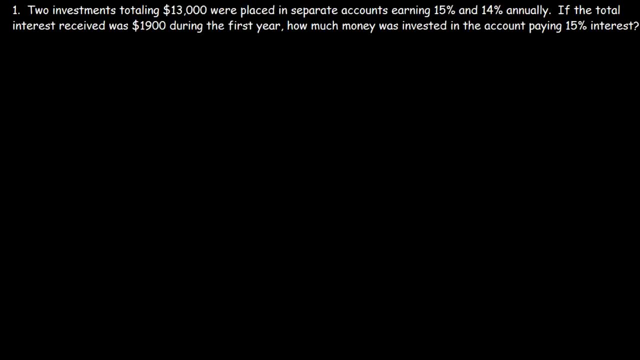 earning 15% and 14% annually. If the total interest received was 1,900 during the first year, how much money was invested in the account paying 15% interest? Well, let's write an equation. Let's say that x. 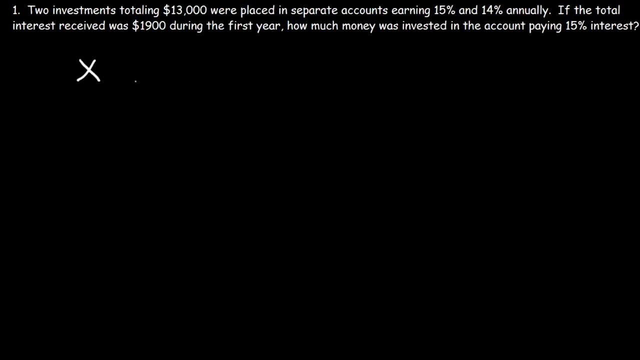 is the amount of money paid or placed in the first account And y is for the other account. x plus y has to add up to the total investment. So y plus y has to add up to the total investment. Now the total interest is 1,900.. 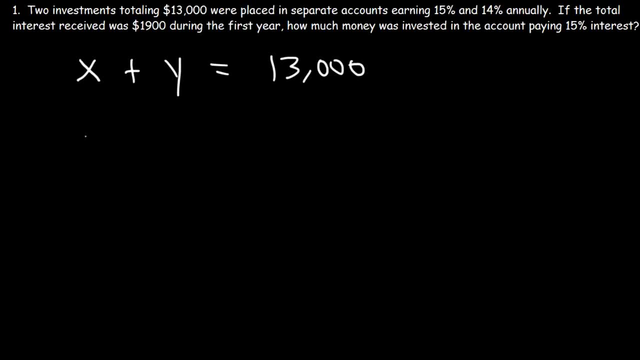 So the first account which x amount of money was placed in. let's say that account paid 15% interest. 15% as the decimal is 0.15.. To convert a percentage into a decimal, divide by 100.. 14 divided by 100 is 0.14.. 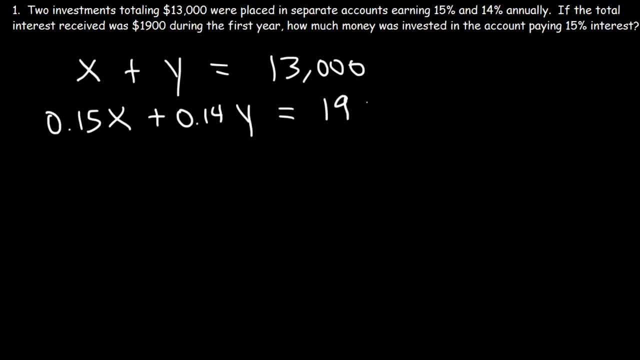 So this should equal 1,900, the total interest received from both accounts. So now that we have a system of equations, we can solve it. Whenever you have two variables, you need two equations to solve those two variables. And since we have decimals, 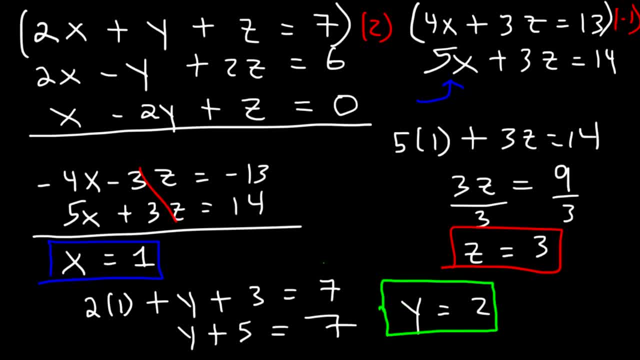 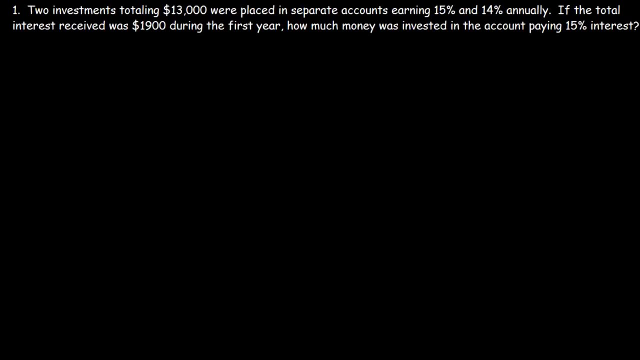 So we can write the answer like this: 1 comma, 2 comma 3.. x, y is z. So that's it for that problem. Now let's work on some word problems. Two investments totaling 13,000 were placed in separate accounts. 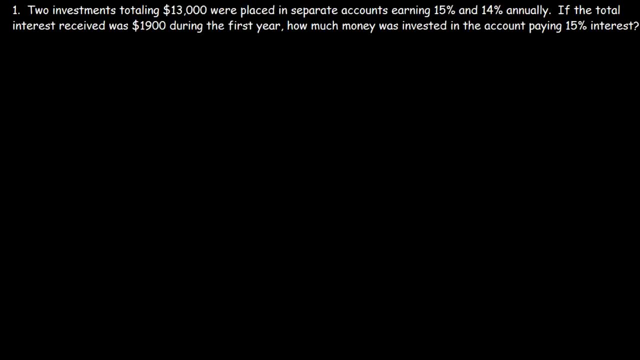 earning 15% and 14% annually. If the total interest received was 1,900 during the first year, how much money was invested in the account paying 15% interest? Well, let's write an equation. Let's say that x. 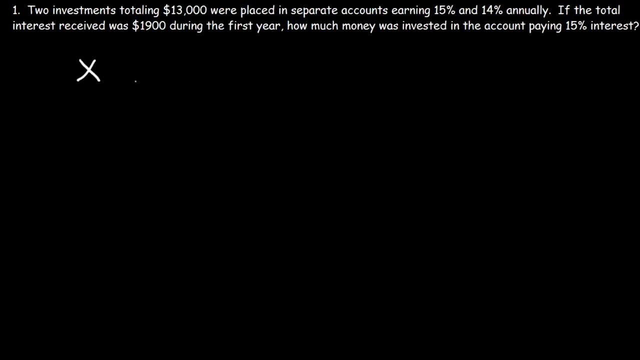 is the amount of money paid or placed in the first account And y is for the other account. x plus y has to add up to the total investment. So y plus y has to add up to the total investment. Now the total interest is 1,900.. 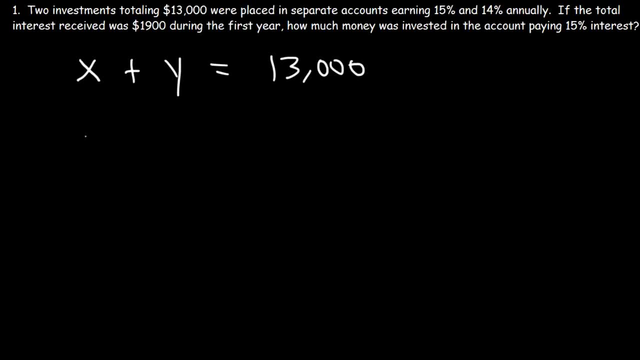 So the first account which x amount of money was placed in. let's say that account paid 15% interest. 15% as the decimal is 0.15.. To convert a percentage into a decimal, divide by 100.. 14 divided by 100 is 0.14.. 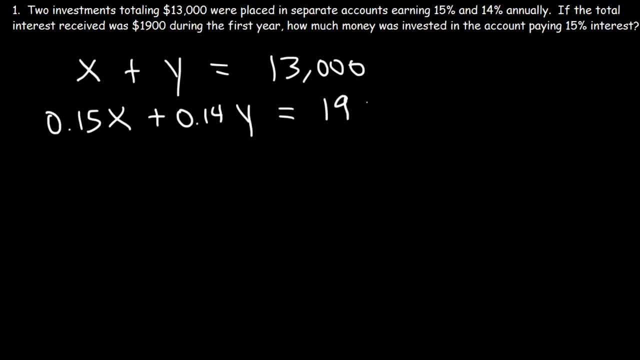 So this should equal 1,900, the total interest received from both accounts. So now that we have a system of equations, we can solve it. Whenever you have two variables, you need two equations to solve those two variables. And since we have decimals, 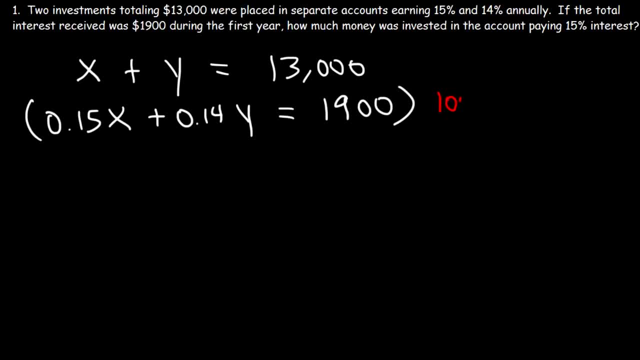 let's multiply the second equation by 100.. 0.15 times 100 is 15.. And 0.14 times 100 is 14.. 1,900 times 100 is 190,000.. Just add two zeros. 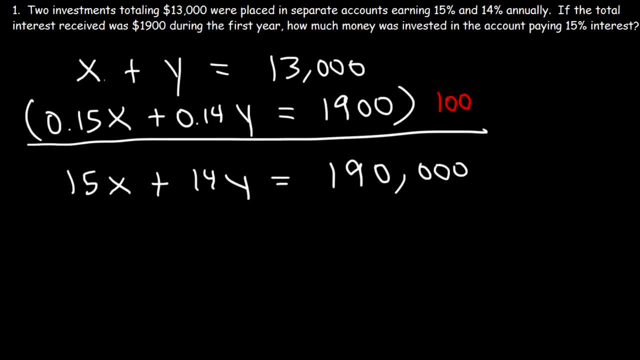 Now let's solve this by elimination. Let's cancel the y variable, So let's multiply the first equation by negative 14.. So we're going to have negative 14x minus 14y And then 13,000 times negative 14. 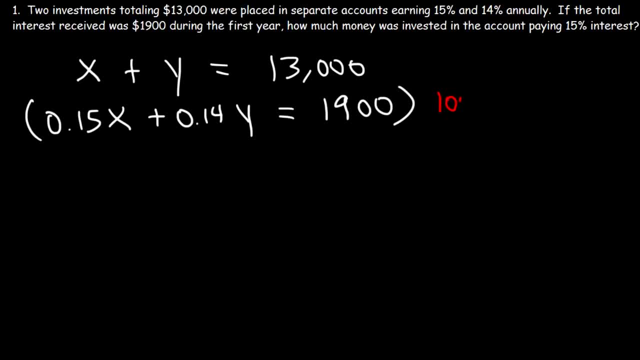 let's multiply the second equation by 100.. 0.15 times 100 is 15.. And 0.14 times 100 is 14.. 1,900 times 100 is 190,000.. Just add two zeros. 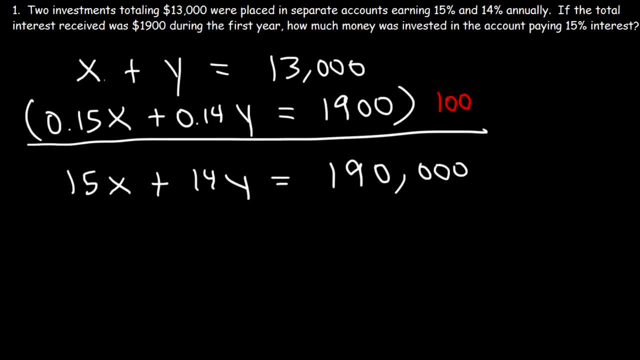 Now let's solve this by elimination. Let's cancel the y variable, So let's multiply the first equation by negative 14.. So we're going to have negative 14x minus 14y And then 13,000 times negative 14. 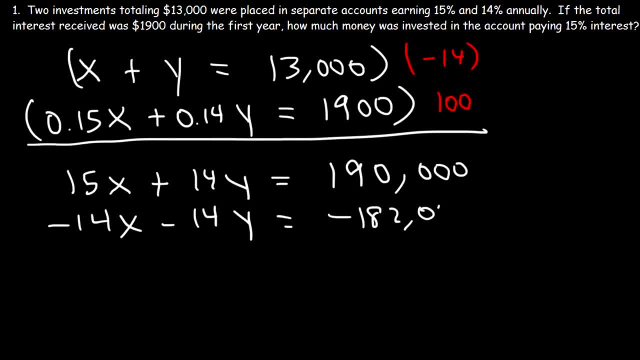 is negative 182,000.. Now let's add the two equations: 15 minus 14 is x, The y's will cancel, And 190,000 minus 182,000 is 8,000.. So that's how much money. 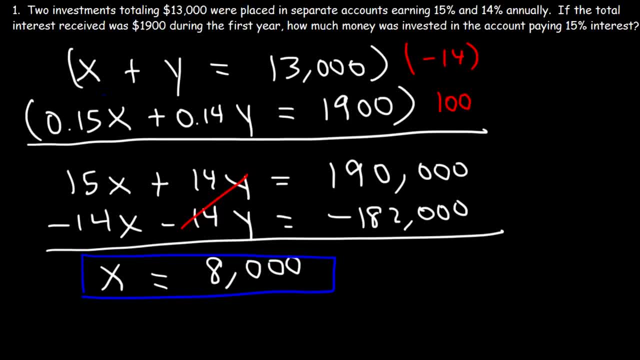 was invested in the account paying 15% interest because x is associated with 15%. Now the total investment is 13,000, which means that 5,000 was placed in the other account. So that's the account that was paying 14% interest. 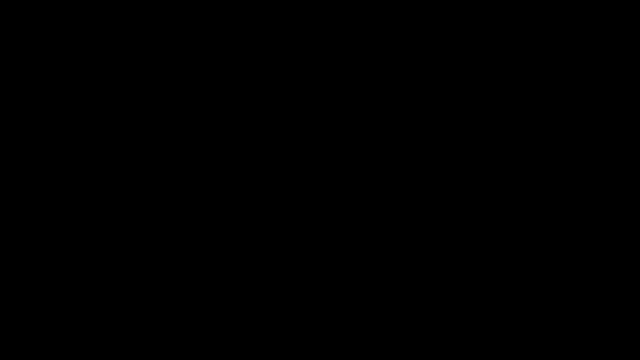 And so that's it for this problem. Now let's make sense of that problem. So 8,000 was placed in the first account, which paid 15% interest. 15% of 8,000, if you multiply these two numbers, is 1,200.. 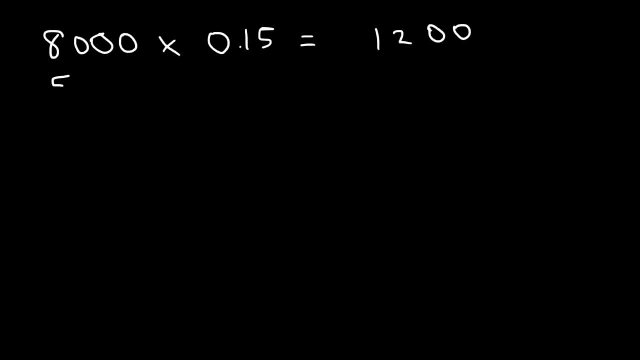 So the first account earned 1,200 in interest alone. Now the second account received $5,000 and was paying 14% interest. So 5,000 times .14 is 700.. So that account received $700 in interest for that year. 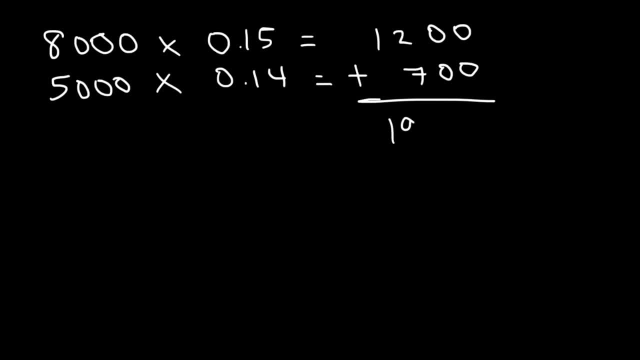 The total interest is 1,200 plus 700, which is 1,900.. So, as you can see, the numbers make sense: If 5 apples and 8 bananas cost $6.55, and if 9 apples and 7 bananas, 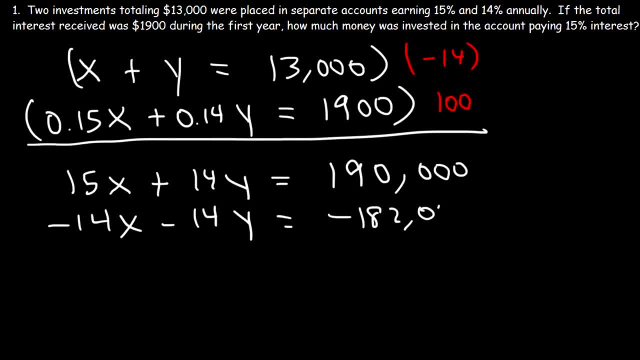 is negative 182,000.. Now let's add the two equations: 15 minus 14 is x, The y's will cancel, And 190,000 minus 182,000 is 8,000.. So that's how much money. 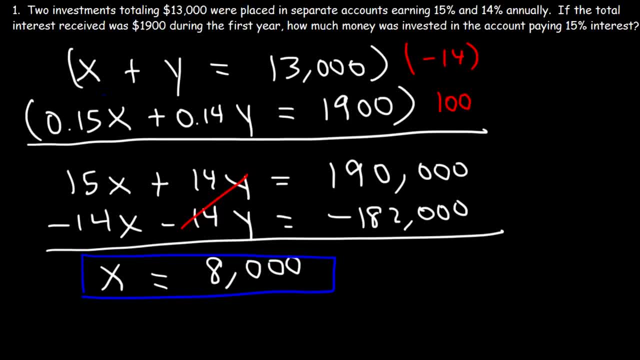 was invested in the account paying 15% interest because x is associated with 15%. Now the total investment is 13,000, which means that 5,000 was placed in the other account. So that's the account that was paying 14% interest. 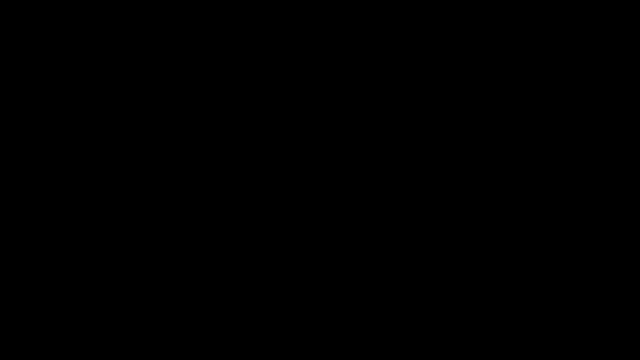 And so that's it for this problem. Now let's make sense of that problem. So 8,000 was placed in the first account, which paid 15% interest. 15% of 8,000, if you multiply these two numbers, is 1,200.. 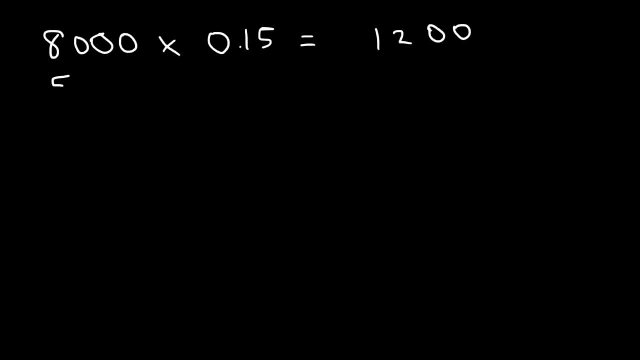 So the first account earned 1,200 in interest alone. Now the second account received $5,000 and was paying 14% interest. So 5,000 times 0.14 is 700.. So that account received $700 in interest for that year. 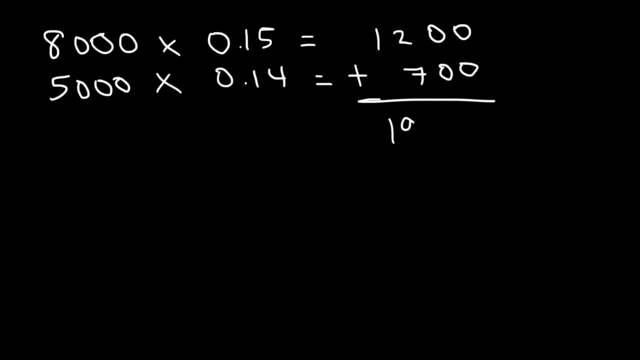 The total interest is 1,200 plus 700, which is 1,900.. So, as you can see, the numbers make sense. If 5 apples and 8 bananas cost $6.55, and if 9 apples and 7 bananas, 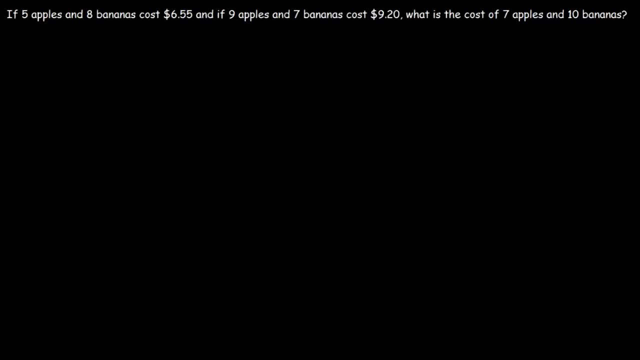 cost $9.20,. what is the cost of 7 apples and 10 bananas? We have two variables: apples and bananas. We'll use A and B to represent those variables. So we need to write two equations If we could find the value of. 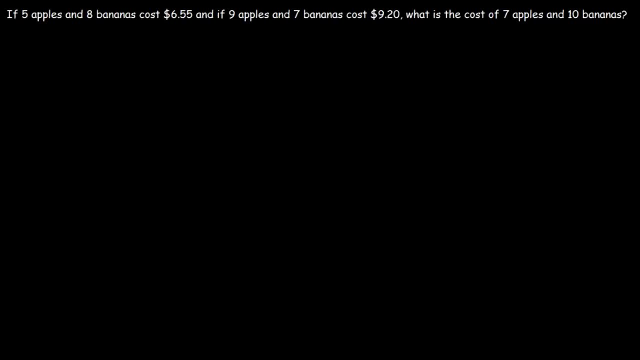 1 apple and 1 banana. then we could find the value of 7 apples and 10 bananas, which is the goal of the problem. So the first part of the problem states that 5 apples, or 5a, plus 8 bananas. 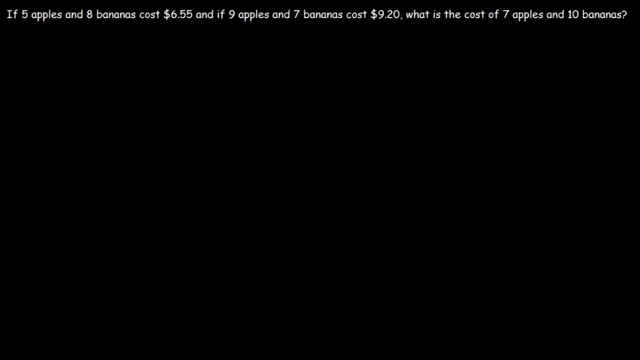 cost $9.20,. what is the cost of 7 apples and 10 bananas? We have two variables: apples and bananas. We'll use A and B to represent those variables. So we need to write two equations If we could find the value of. 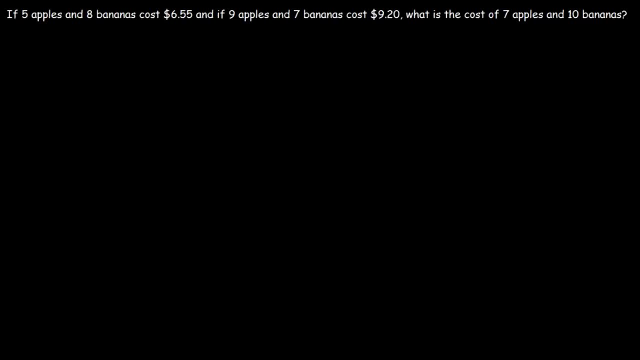 1 apple and 1 banana. then we could find the value of 7 apples and 10 bananas, which is the goal of the problem. So the first part of the problem states that 5 apples, or 5A, plus 8 bananas. 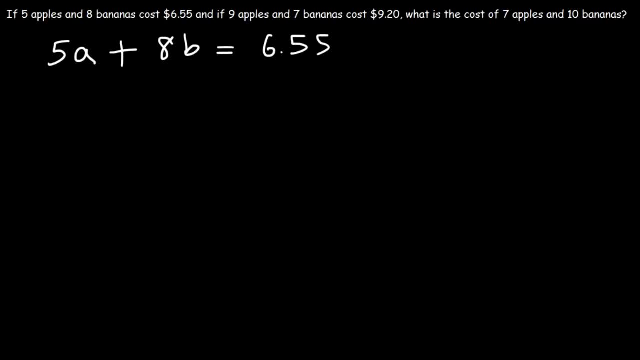 has a cost of $6.55.. So 5A plus 8B equals 6.55.. 9 apples and 7 bananas cost $9.20.. Let's use these two equations to find the value of each apple and each banana. 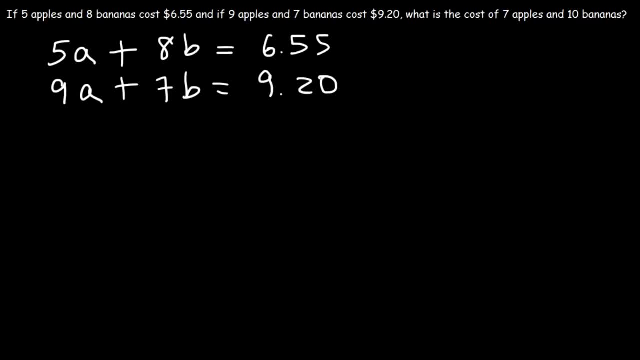 So what do you think we should do Now? if you want to, we can get rid of the decimal. We can multiply both sides by 100, but we don't have to. Let's multiply the first equation by negative 7 to get rid of B. 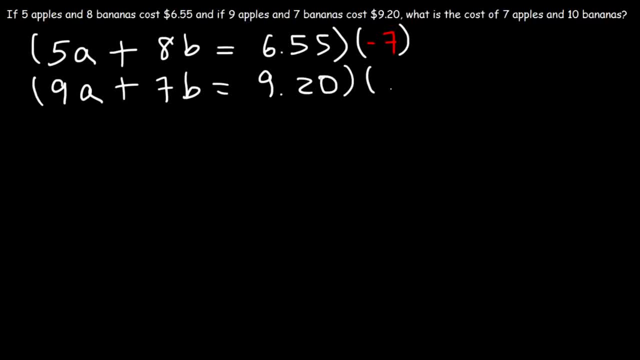 And let's multiply the second equation by positive 8.. We want to get 56B. 5A times negative. 7 is going to be negative. 35A. 8B times negative. 7 is negative. 56B And 6.55. 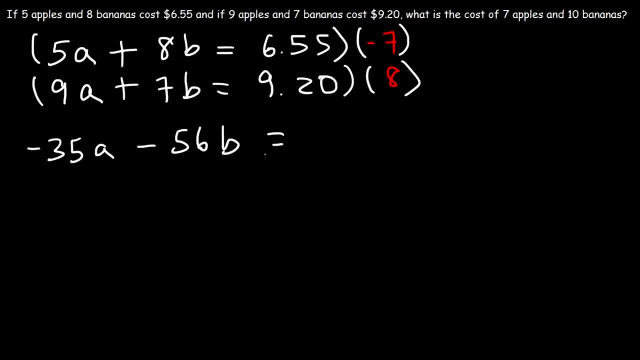 times negative 7, that's going to be negative 45.85.. 9A times 8 is 72A. 7B times 8 is positive 56B. 9.20 times 8 is 73.60.. 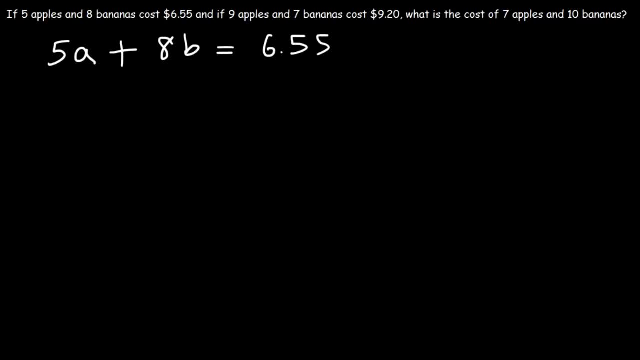 has a cost of $6.55.. So 5a plus 8b equals 6.55.. 9 apples and 7 bananas cost $9.20.. Let's use these two equations to find the value of each apple and each banana. 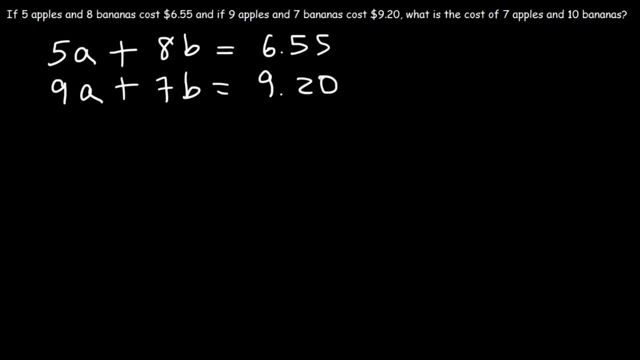 So what do you think we should do Now? if you want to, we can get rid of the decimal. We can multiply both sides by 100, but we don't have to. Let's multiply the first equation by a negative 7. 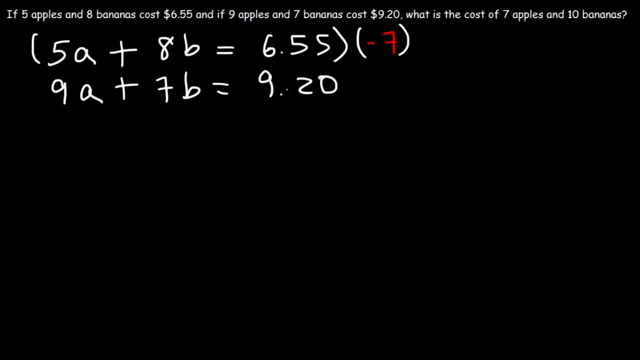 to get rid of B, And let's multiply the second equation by a positive 8.. We want to get 56b. 5a times negative, 7 is going to be negative. 35a. 8b times negative: 7 is negative 56b. 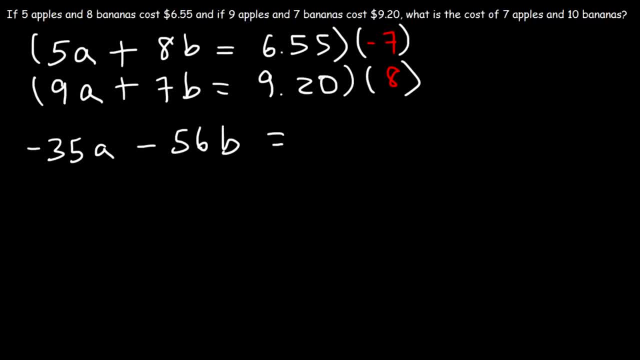 And 6.55 times negative 7, that's going to be negative 45.85.. 9a times 8 is 72a. 7b times 8 is positive 56b. 9.20 times 8 is 73.60.. 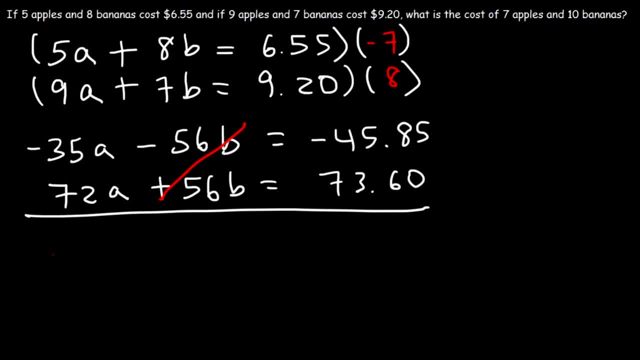 Now let's add the two equations: Negative 35 plus 72,, that's going to be positive 37, or 37a. Negative 45.85 plus 73.60,, that's 27.75.. So now a is going to be 27.75. 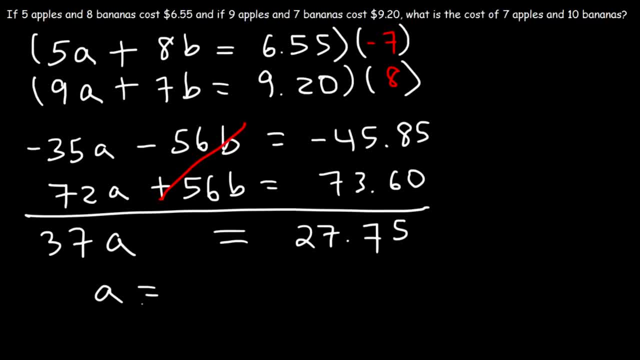 divided by 37.. So the cost of each apple is 75 cents. Now let's use the first equation in its unmodified form to find b. So 5 times 0.75 plus 8b is equal to 6.55. 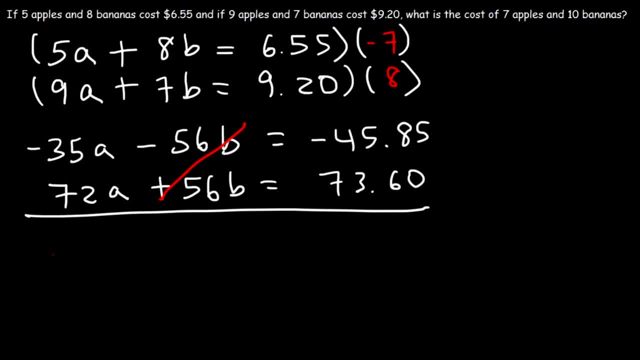 Now let's add the two equations: Negative 35 plus 72,, that's going to be positive 37, or 37A. Negative 45.85 plus 73.60,, that's 27.75.. So now A is going to be 27.75. 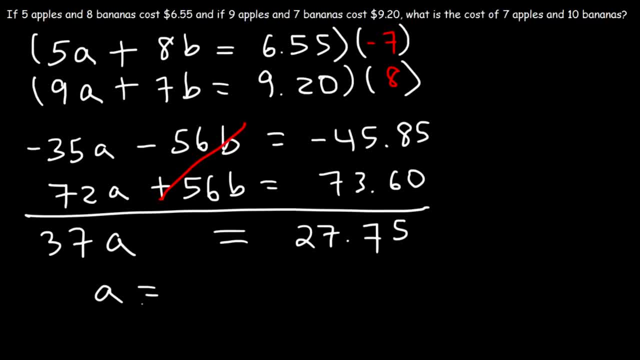 divided by 37.. So the cost of each apple is 75 cents. Now let's use the first equation in its unmodified form to find B. So 5 times 0.75 plus 8B is equal to 6.55. 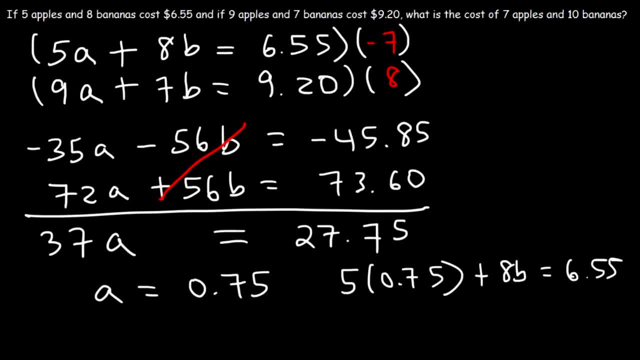 So 5 times 0.75 is 3.75.. Now let's subtract both sides by 3.75.. So 6.55 minus 3.75, that's equal to 2.8.. And B is going to be 2.8. 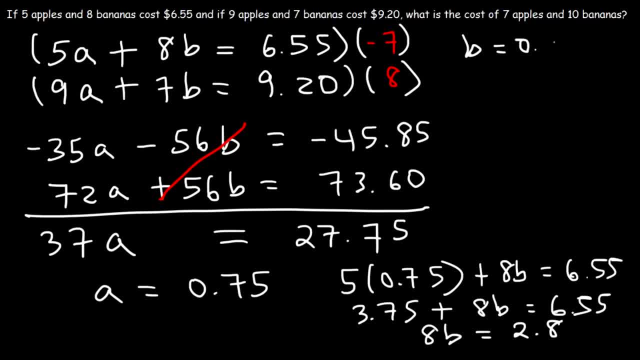 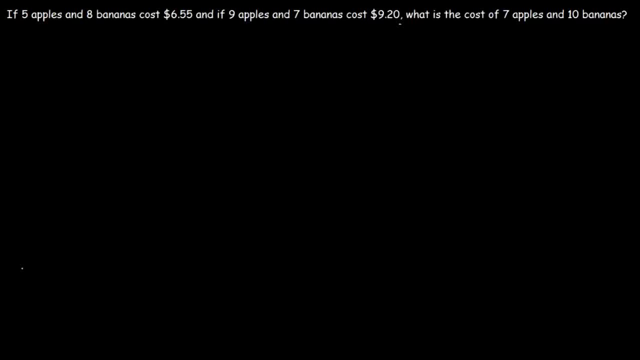 divided by 8, which is 35 cents. So now we have the cost of every apple and every banana. So the cost of a single apple is 75 cents And the cost of a single banana is 35 cents. So now we can find the value. 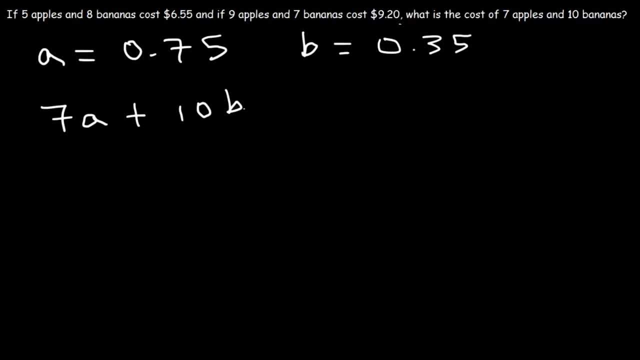 of 7 apples and 10 bananas, So it's going to be 7 times 75 cents, plus 10 times 35 cents. 7 times 0.75 is 5 dollars and 25 cents 10 times 0.35,. 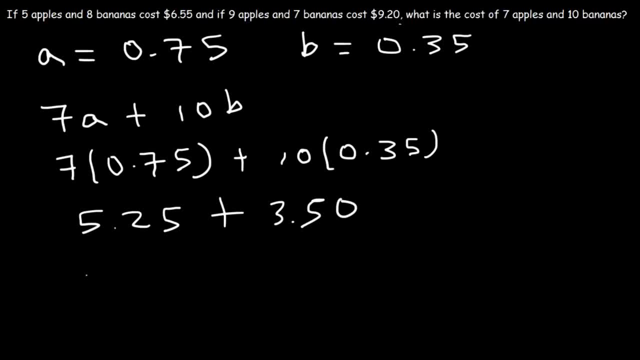 you just got to move the decimal. that's 3 dollars and 50 cents. So if we add this, this should be 8.75.. So that's the cost of 7 apples and 10 bananas. It's 8 dollars and 75 cents.